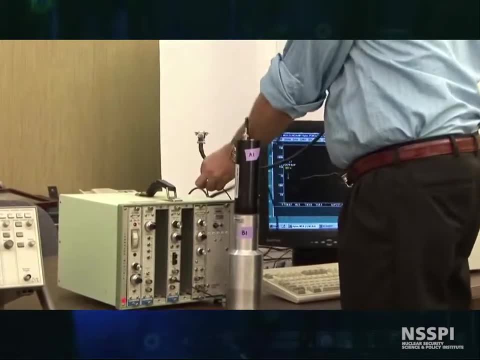 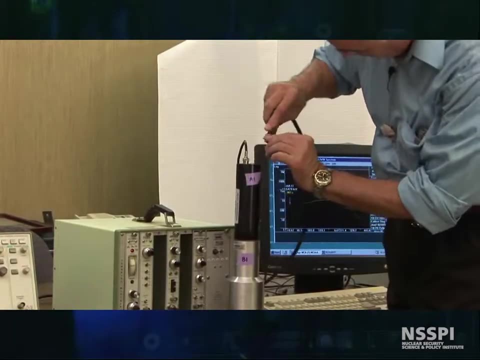 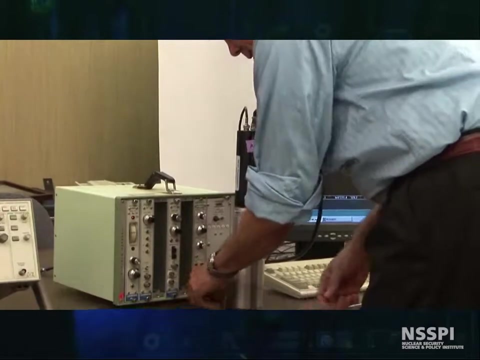 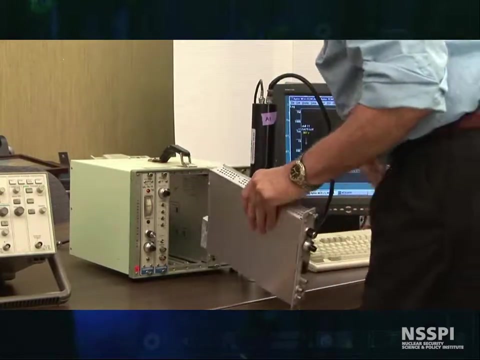 connector that supplies power to the tube. This goes here, And there are several ways to do this: 3. Connect the connector to the tube. can just go around back and hook it up, but you won't see very much, So I can pull this. 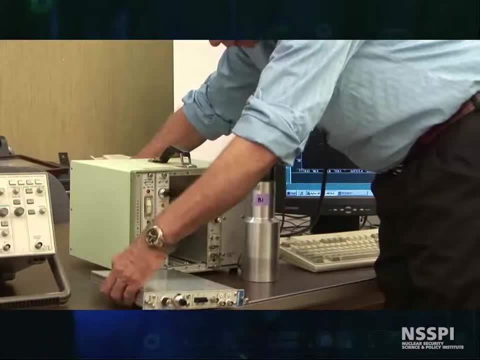 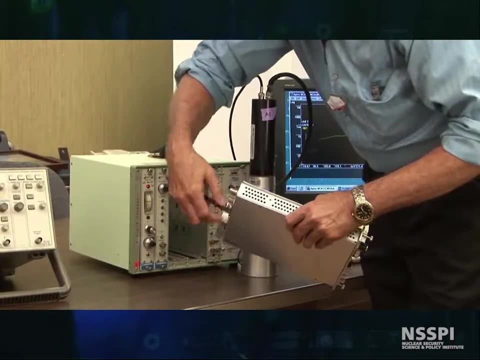 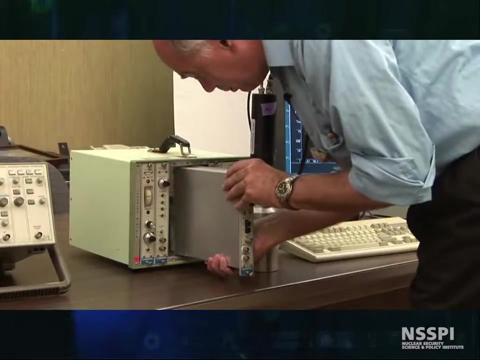 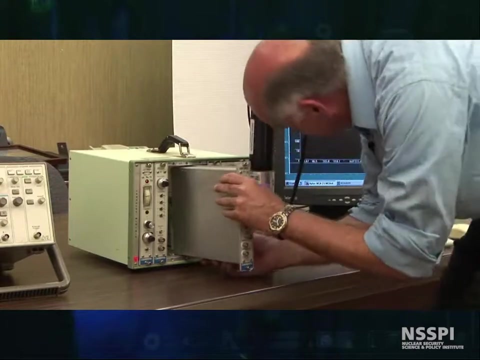 out of the NEM bin, feed this through and it hooks up in the back right here, And this is feeds the preamps. This is traditionally how it's done. The preamp that I used before the power to hit was fed the same way. There's little slots that this fits in which I will. 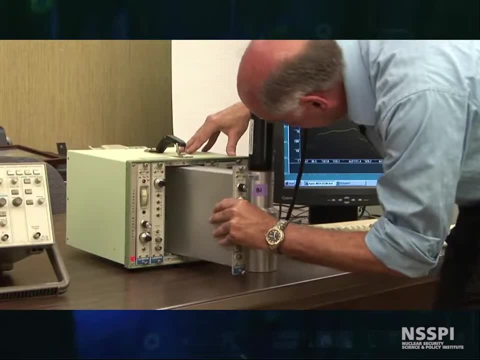 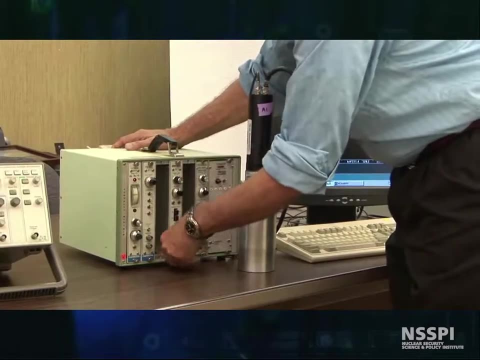 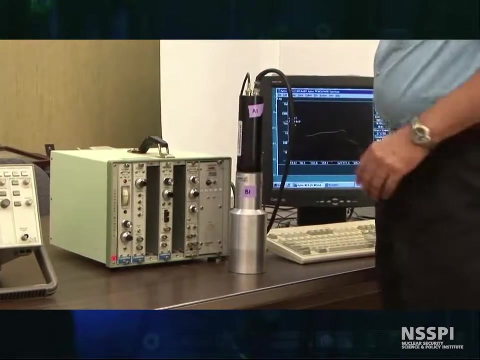 get in there sooner or later. And now I can turn on the power to the NEM for the ainsiинов stallage, That kimchi chowder. The NEM is very yummy and the tea pack isn't to be considered hearty. And now I started to prepare the favorite pet. 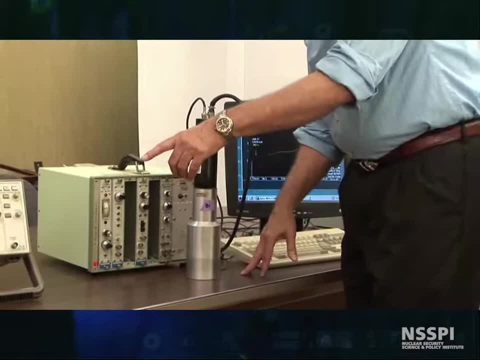 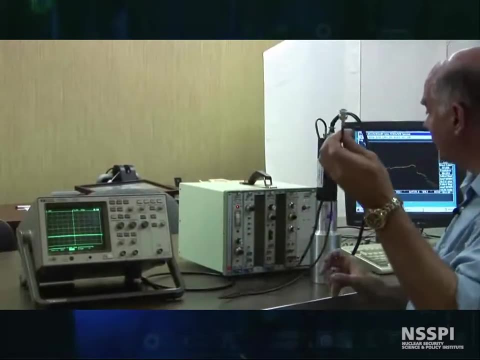 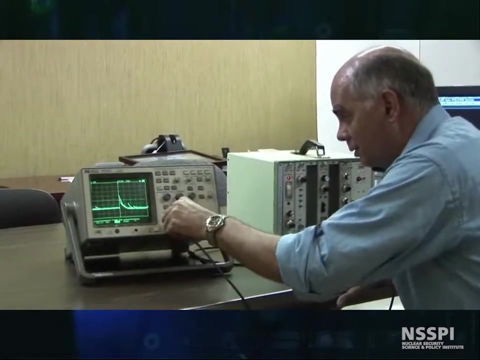 the sodium iodide detector. Let's move over here and look at what the pulses look like coming out of the detector. Okay, so we can take the signal from the sodium iodide. We can go into our friend, the O-scope, and there they are. We can see the gammas. there They're. 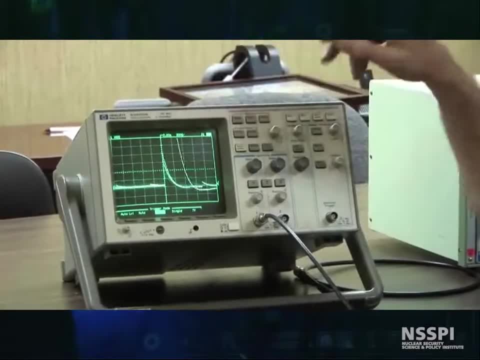 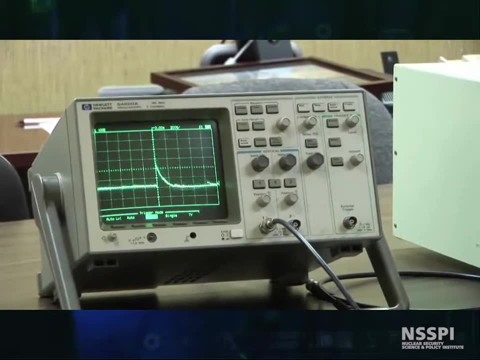 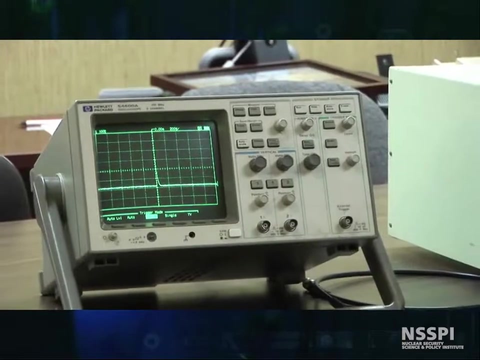 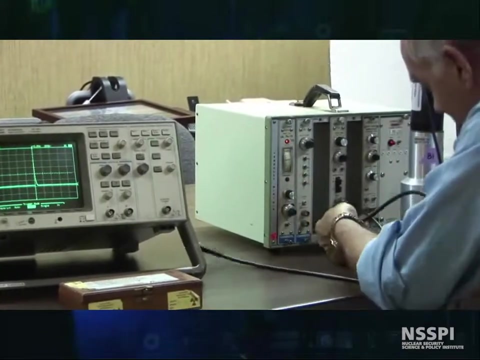 relatively slow pulses. This is set on 200 microseconds, so you can see it takes quite a while for them to come down. Let's see, can I slow it down? Nope, So from here we're going to take our signal and go into our amplifier and then we're going to take out of our amplifier. 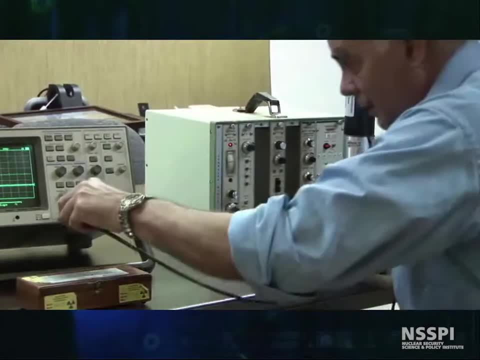 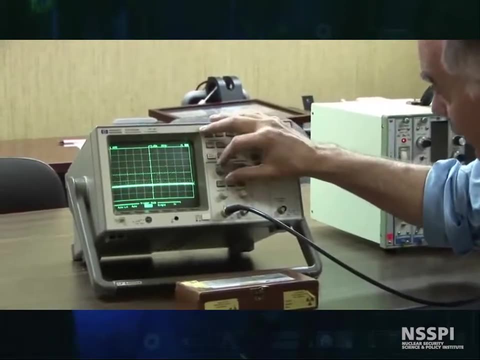 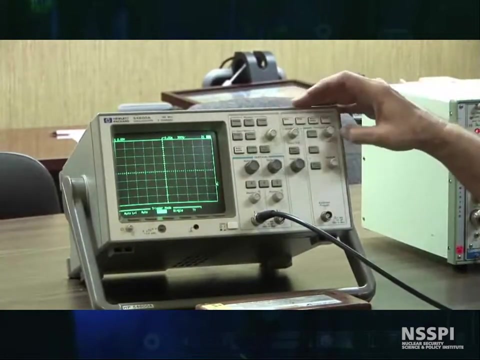 and let's see what happens, What it looks like coming out of the amplifier. Oh my gosh, they're fast, Okay, and they're bigger. So I'm going to go up to a couple of volts. Let's change the level here There. 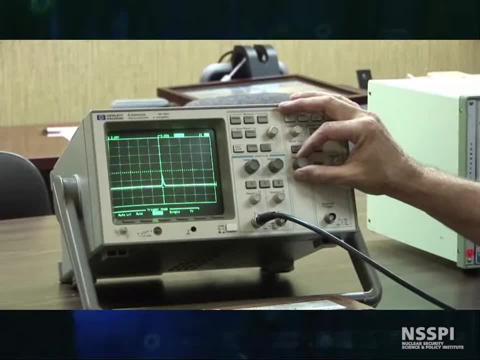 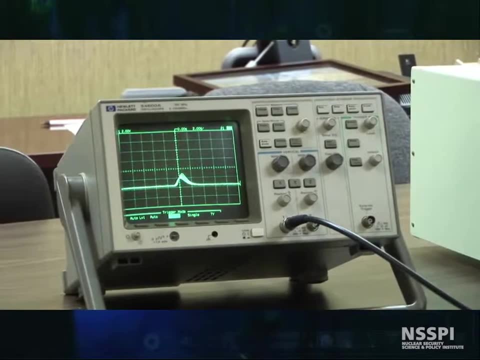 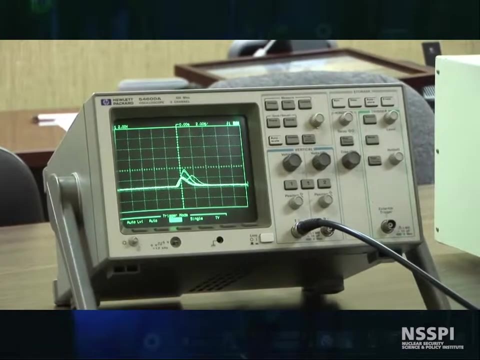 they are. We're going to spread them out and there's our gamma signals And it looks a whole lot like the same signal that came out of our BSL And the signal is coming out of these two F3 tubes and that's kind of the joy of NIMBENs.